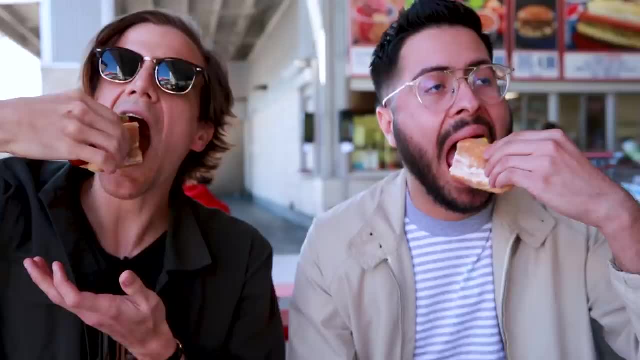 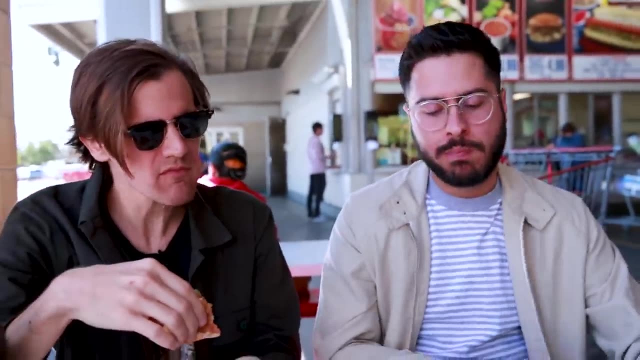 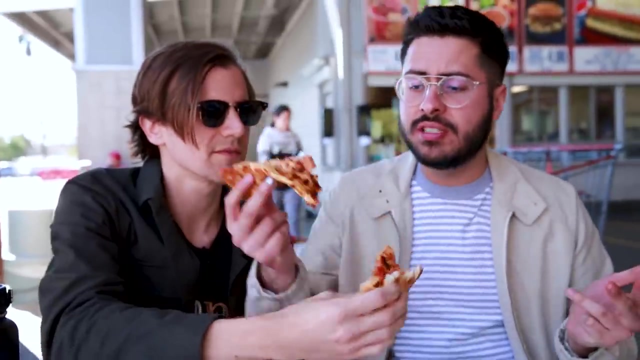 What kind of pizza? where'd you eat your pizza from dude Rome Stadium dog, classic stadium dog. This is actually better than a lot of hot dogs I've had for more money If you are gonna bring a date to Costco. 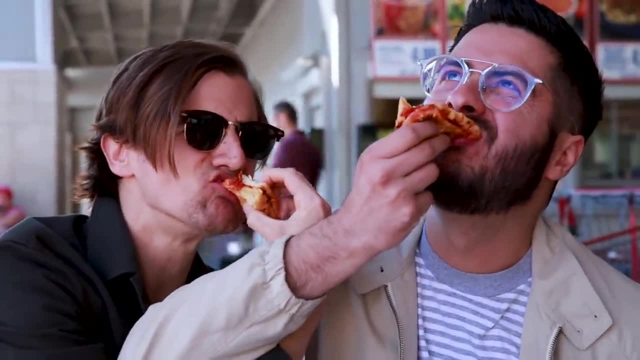 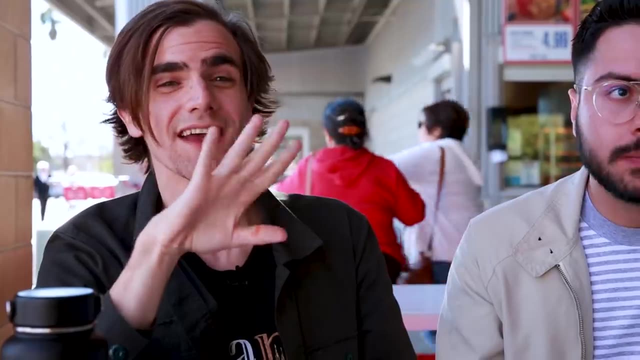 this is how you gotta be eating it. You don't like it. It reminds me of gas station pizza And I like gas station pizza. So it does remind me of gas station pizza. Maybe if it had a topping it would be better. 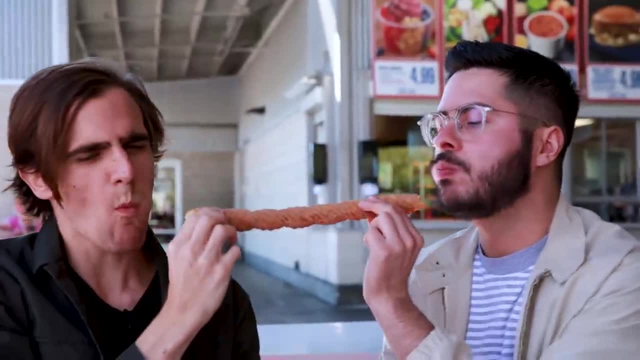 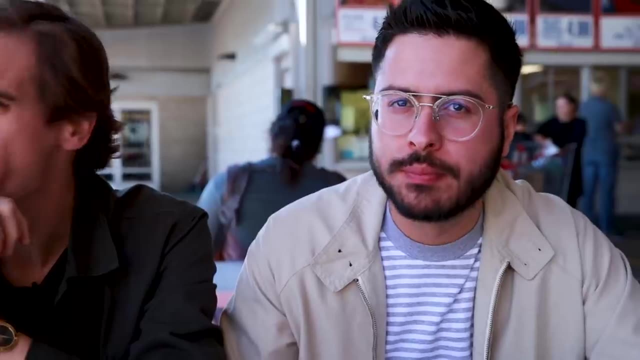 I like the pizza. it's good. One to five. as far as food, I give it a 4.5.. I'll give this a taste of three. This is like a okay, cheap, Questionable food, Like there's other places where I would be like. 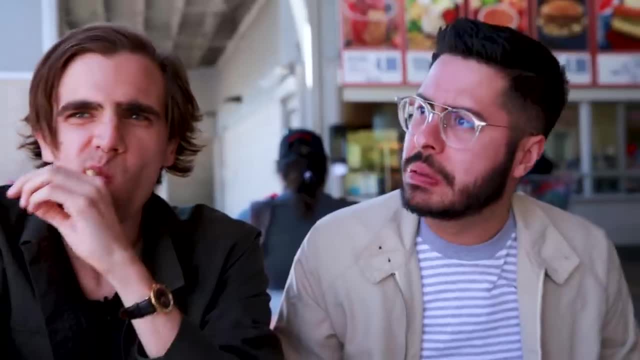 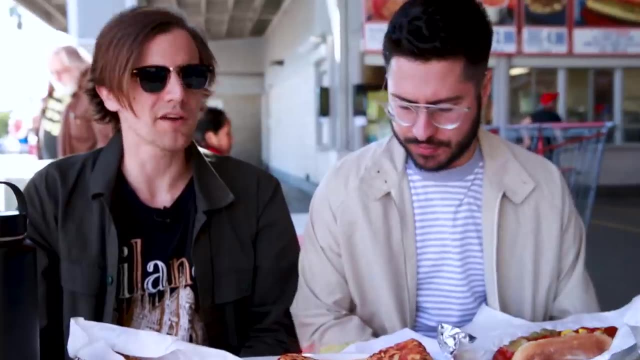 No, this is good. Yeah, What Name a better place? 7-Eleven? No, you got me up. That is disrespectful to Costco. Ordering was so easy and simple and fast. I mean, Just pull up order, swipe your card. 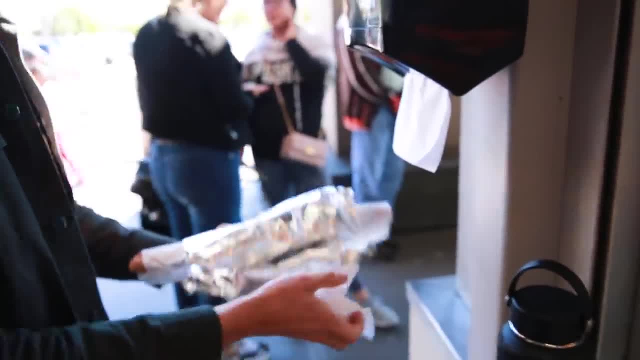 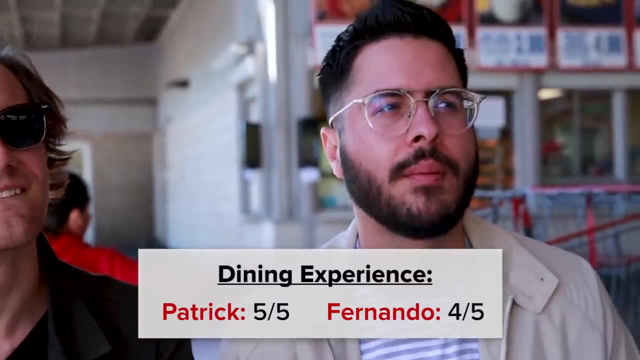 Yeah, And they hand you the food. It's really nuts how they do it here. A quick experience: I give this experience a five. I give this parking lot restaurant a four star On ambience and experience. the table had mustard when we sat down, but 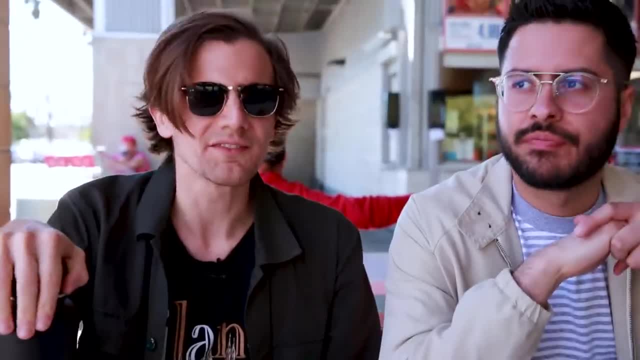 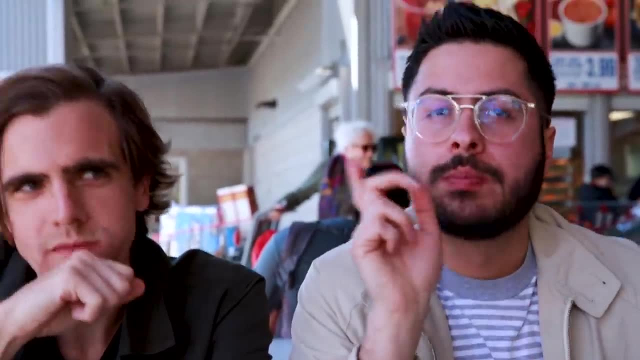 that's totally fine because you're just quick on the go. you know The value on this was insane: Five Less than $5 for all this stuff. it's a five. If I have kids, I will bring them here, go inside, do my grocery shopping without. 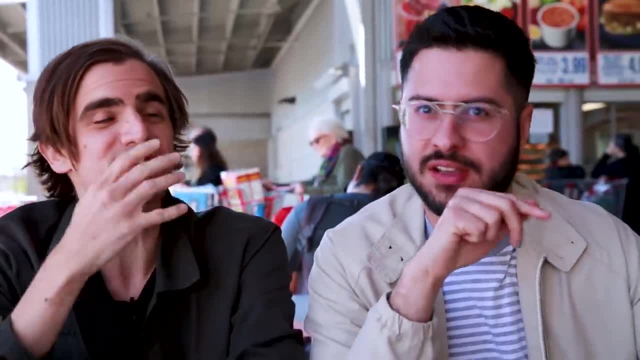 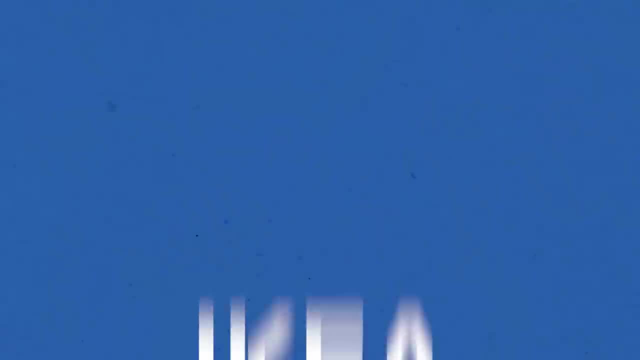 them. buy them like $20 worth of pizza. You're just gonna leave your kids out here. You're just gonna leave. Listen, okay, maybe I won't leave them. I'll give them a phone First. presentation and ambience is much better here, I feel. 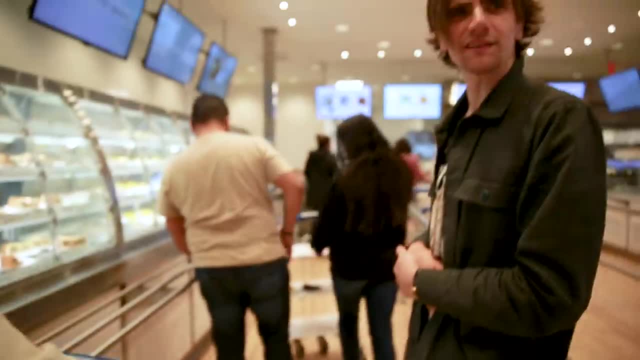 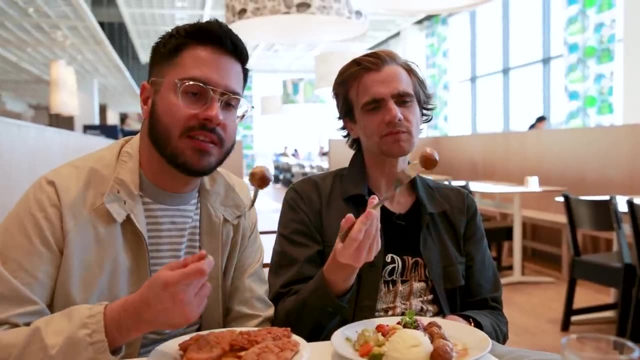 Yeah, this is like this rules. Yeah, I love the wood aesthetic. It's much more like homey kitchen, like I want to like sit and like have something that grandma made for me. you know, We'll go to town with the classic, the Swedish meatballs. 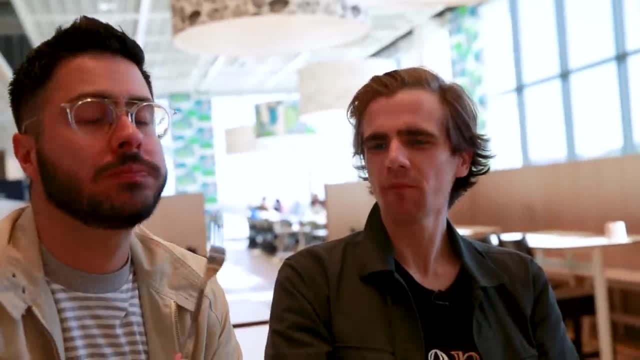 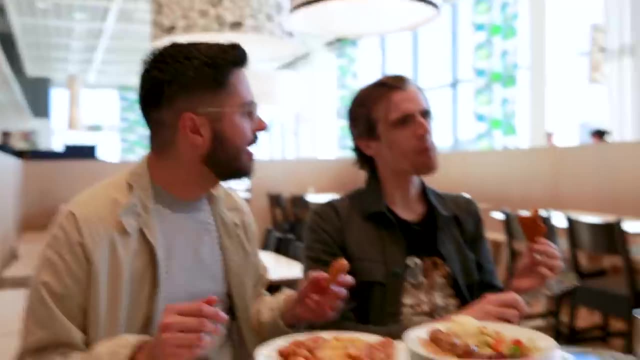 Cheers, Mm-hm, that was really good. Yeah, that was really nice. First impression This: You haven't done a taste test in a long time. huh, It's been a whole month since you haven't been at BuzzFeed and you forgot. 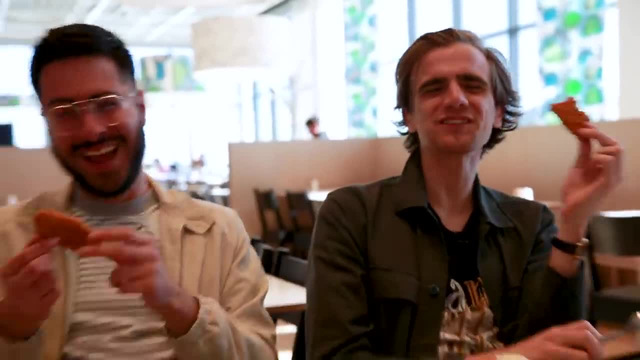 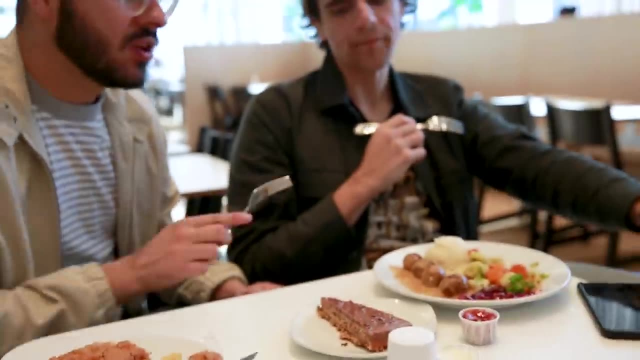 They're good. They're good. Yeah, these are the good ones. Yeah, Mm-hm, Really crunchy and flaky on the outside. it's nice. You're on a diet, right? Yeah, yeah, So this has to be really good in order for. 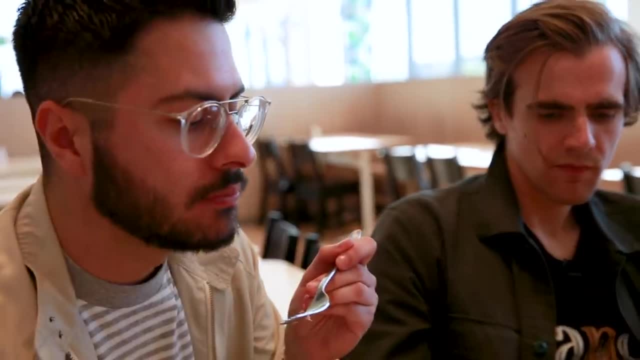 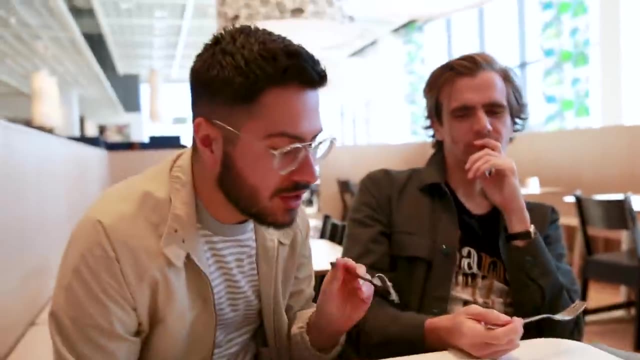 you to really think it's worth breaking your diet. Yeah, totally, Mm, mm-hm, that's good, Mm-hm, Mm, It's good. Yeah, that's good, Mm-hm. These little nuts on top. 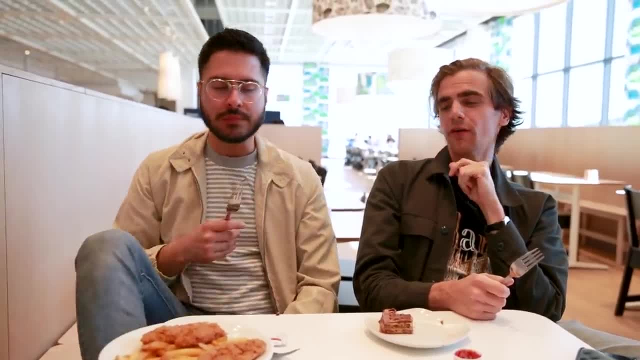 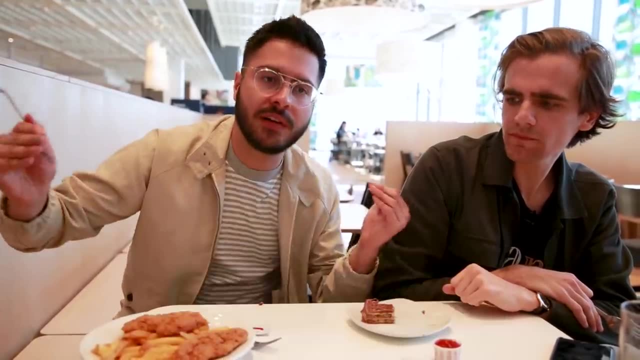 Mm-hm. I'm into that Food pretty good, I'll give it a four. This I will give a 4.5 as well. I think they're both equally good in different spectrums of where you want to get food. 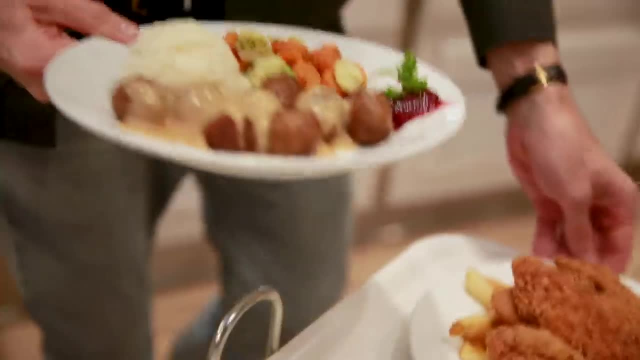 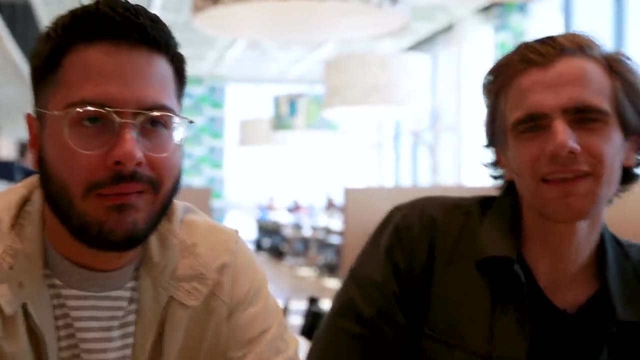 I just gotta say from the moment we walked in, the ambience is definitely an improvement. Yeah, look, was it a little tedious. Yeah, like waiting in the line going down different stations. Not my favorite way to order, to be honest with you, but 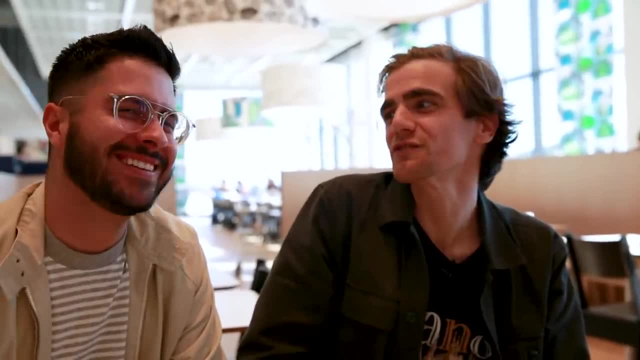 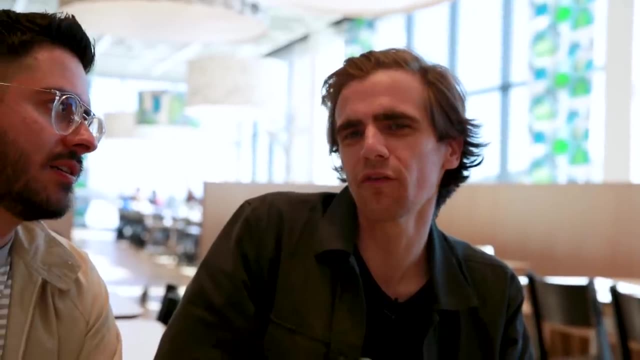 There was one person in front of us. It reminded me of eating at Disneyland, which is a stressful experience. Yeah, for one to five. what would you give Ikea as far as the experience and the ambience? I would say a four and a half. 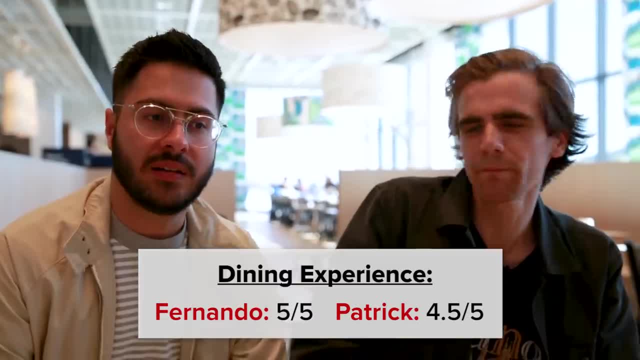 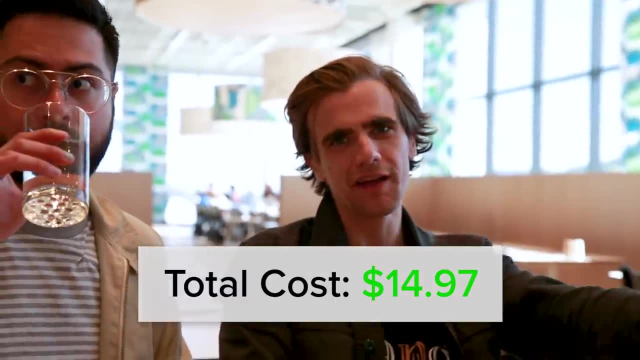 I would give it a five. I think it's a lot cleaner. Big time It's less loud, cuz we're not in a parking lot. Obviously, with one plate we're already spending more than what we spent for three different options at Costco. 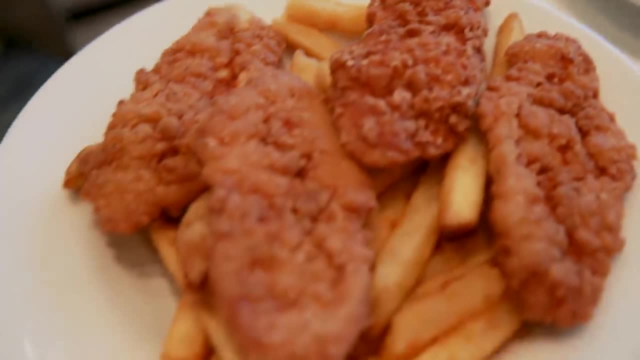 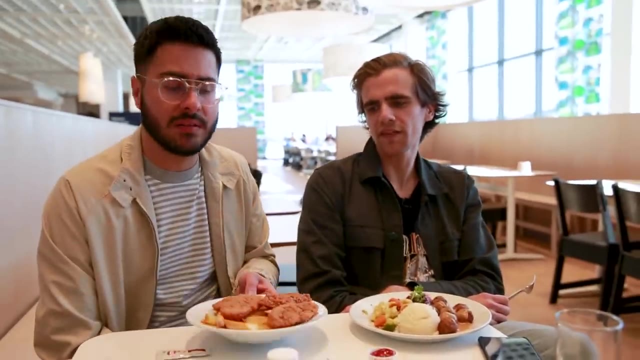 But you got protein, you got your vegetables, you got a little carbs starch. there it's more or less a well-rounded meal. Yeah, I think in value this $6.99,. this is cool, I think. for value I'll give it a three and a half. 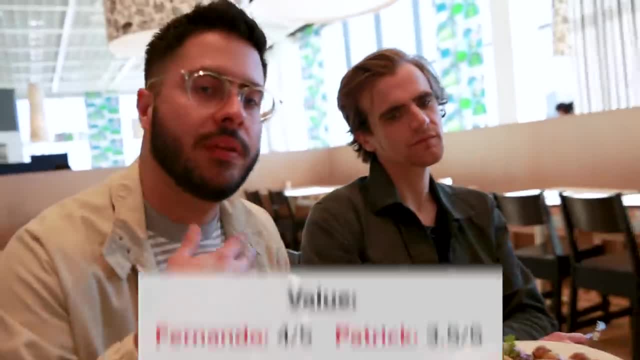 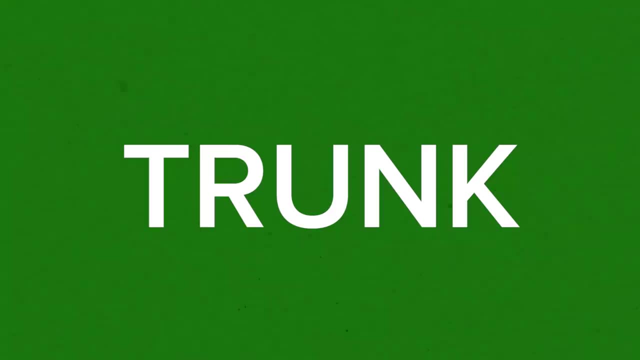 Three and a half, I give it a four for value. The only thing that would make my value go up is if I got more sauces to go with my chicken tenders, Even though I do think Ikea's food was a little bit better. and 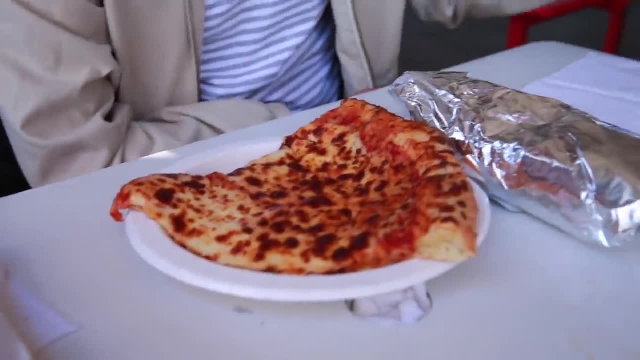 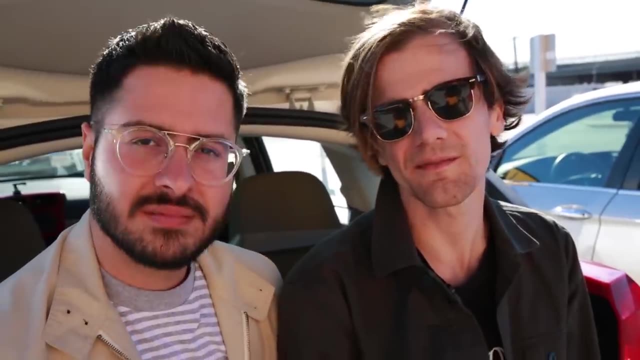 the ambience was better. I think I like Costco better because it delivered on the premise of quick and cheap And eating in a parking lot. I kinda like that. Yeah, it crushed. They were both really good. They're both great. 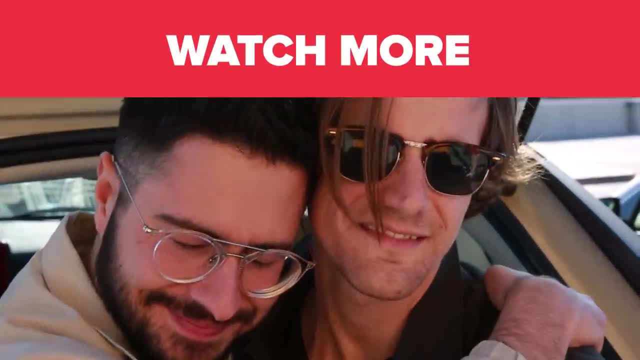 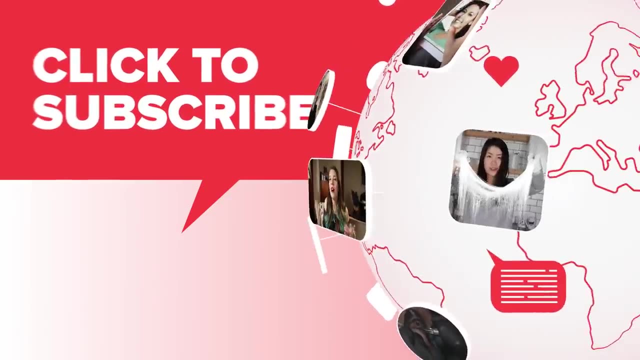 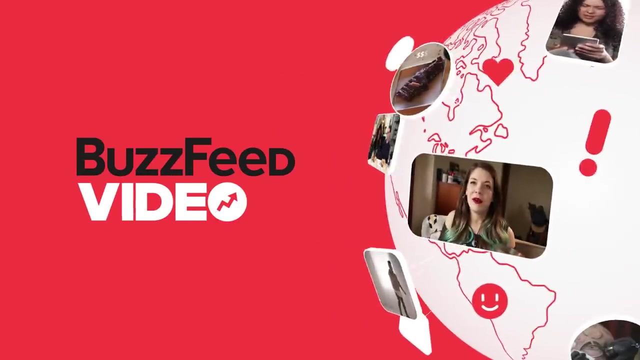 And with a hug. Nothing better than cheap food when you're unemployed, right? Yeah, My friends, I'm gonna be happy if you guys make the next move. If you think you're gonna make a comeback, I'm gonna make sure you make a comeback.